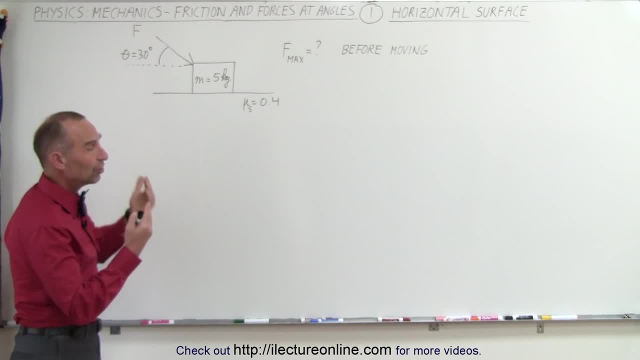 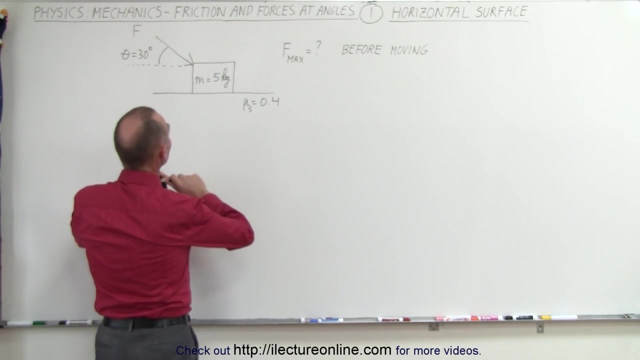 angle of 30 degrees relative to the horizontal. and the question is: what is the maximum force we can apply to the block before the block starts moving? all right, based upon that, let's first determine all of the forces acting on that block. well, first of all, we have the force of gravity acting downward, so we have mg. 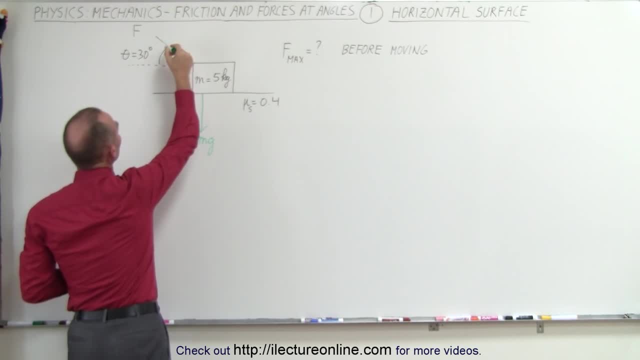 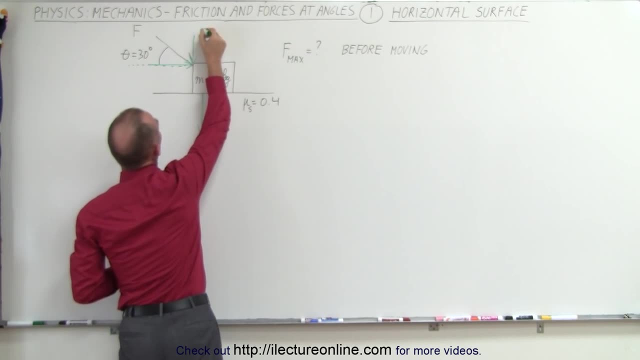 and then we have this force right here which acts as an angle, which means there is a horizontal force and there is a vertical component of that force. so this is the vertical component: f sub y, which is therefore equal to f times d. now we have to be careful, because this would be the opposite side to the angle. so we have 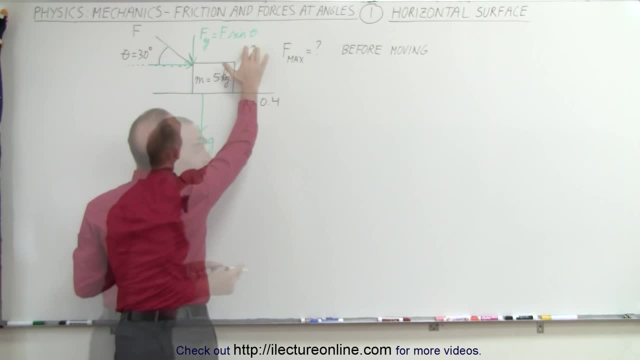 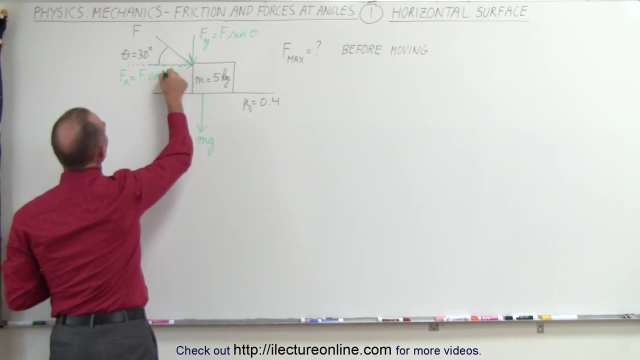 f times the sine of theta for the vertical component and for the horizontal component we have f sub x, which is equal to f times the cosine of theta, so that would be the adjacent side to the angle. now that means that this component is also acting down on the floor. 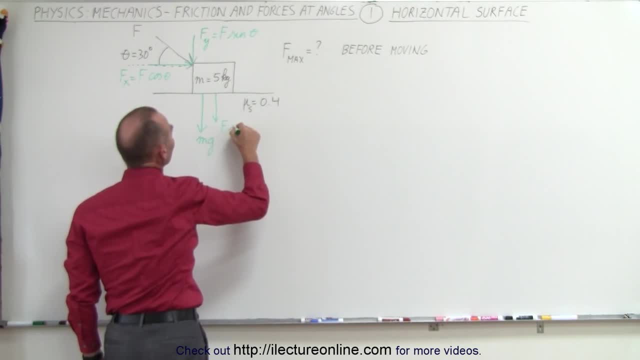 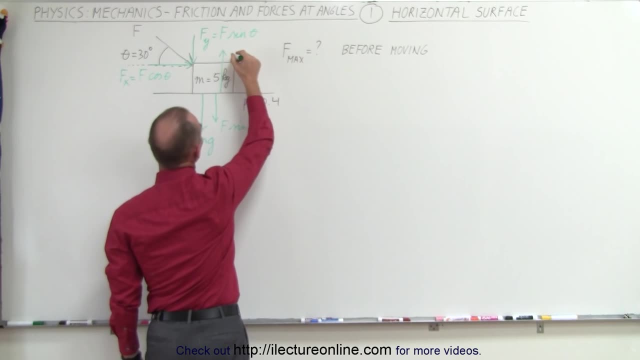 so it's pushing this way with the, with the force f times the sine of theta, and then we have the normal force pushing back, which is going to be the sum of these two forces in the opposite direction. so the normal force is equal to mg plus the f sine theta, which is the vertical component of that. 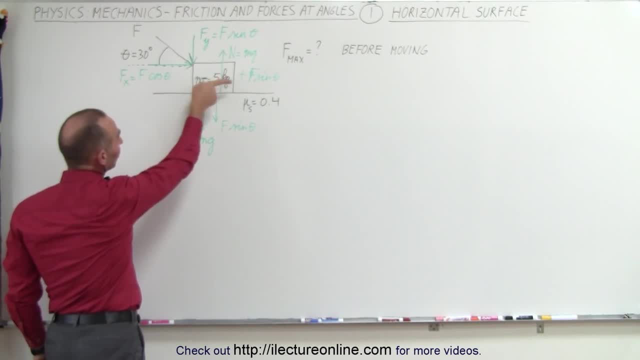 particular force and it's only the horizontal component which is pushing the block to the right. now, the block is not going to move until this horizontal component of the force is greater than the friction force caused by this normal force, The friction force, and let me use a different color for that. 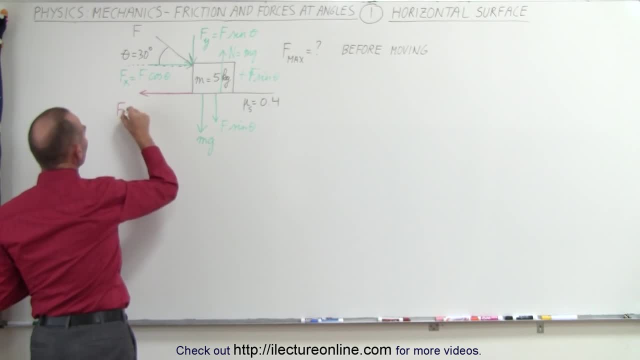 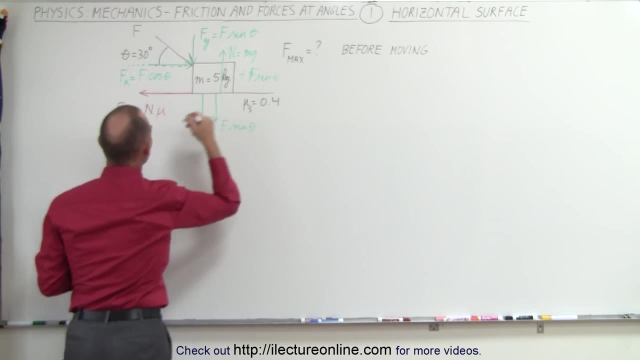 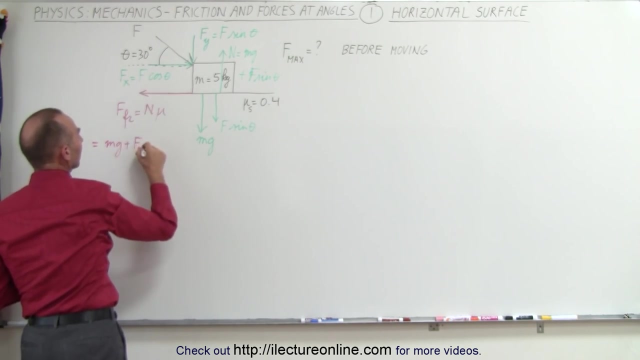 the friction force would be the force pushing this way, force friction, which is equal to the normal force times mu, and of course, in this case the normal force is the sum of these two forces. so that would be equal to mg plus the force applied to the block times the sine. 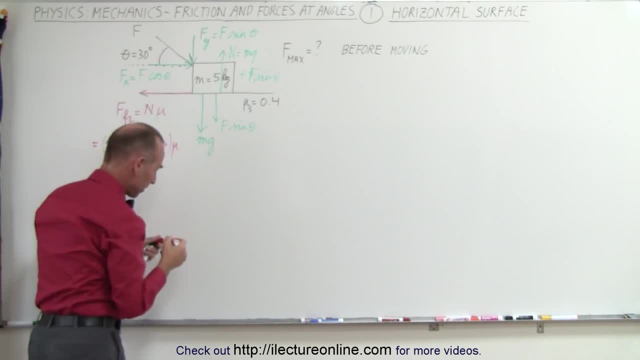 of theta all multiplied times mu. And now we can say that the block will not move until the force in the x-direction, the component in the x-direction, exceeds the friction force, At that point the block will begin to move. so, as long as the force is equal to or less, 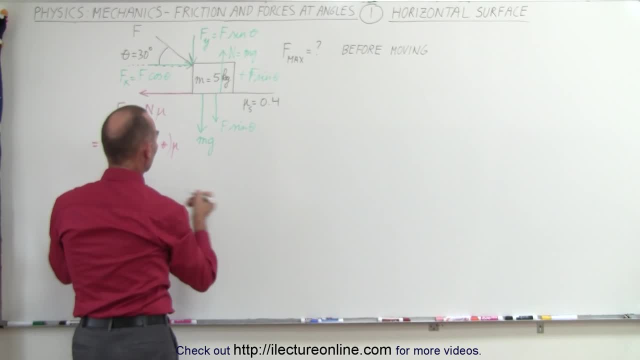 than that force, the block will not move. So we're looking for the F sub X being smaller than the friction force and so, in this case case, small than or equal, to go all the way up to equal to, and the f sub x would be f times the. 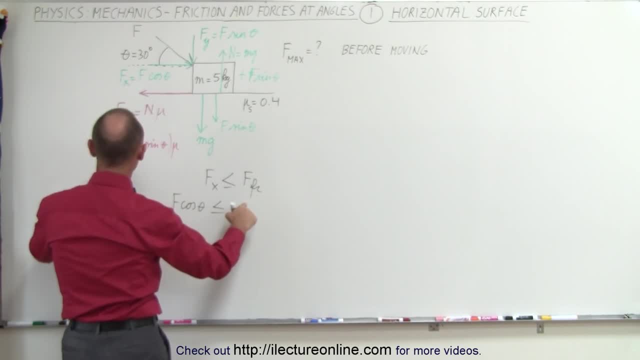 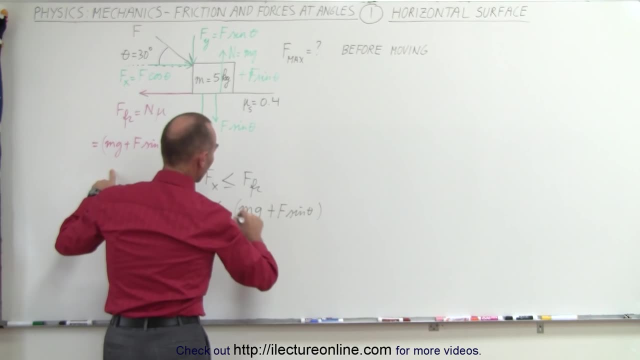 cosine of theta must be smaller, equal to the friction force, which is the normal force, mg plus f times the sine of theta, multiplied times mu, and now all we have to do is solve for f. So first we're going to multiply this through. we get f times the cosine of theta, less than or equal to. 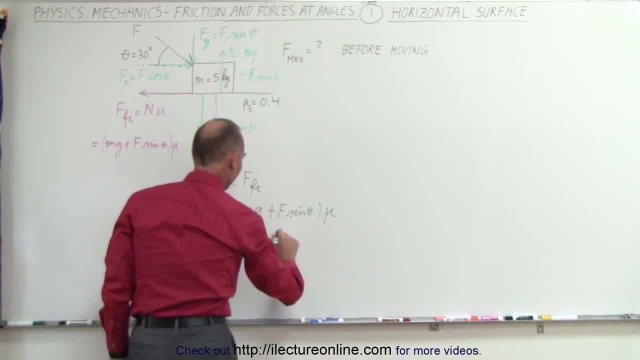 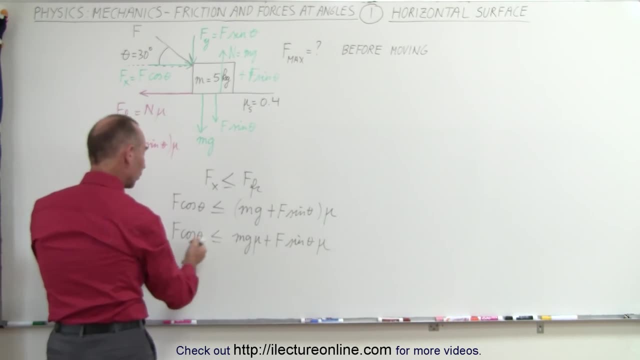 here we have mg mu plus f, sine theta times mu. then we move all the, the components or all the terms that have an f in it to the left side of the equation. so f times the cosine of theta minus f times the sine of theta times mu must be less than or equal to mg mu. 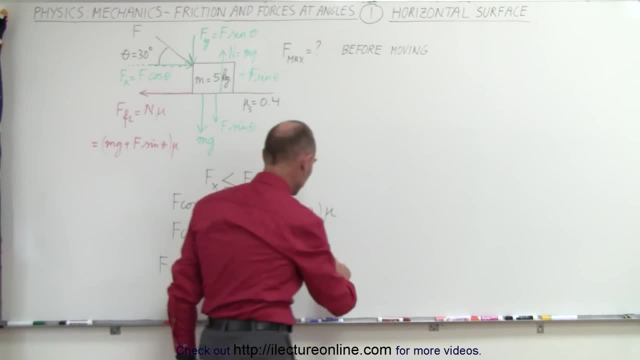 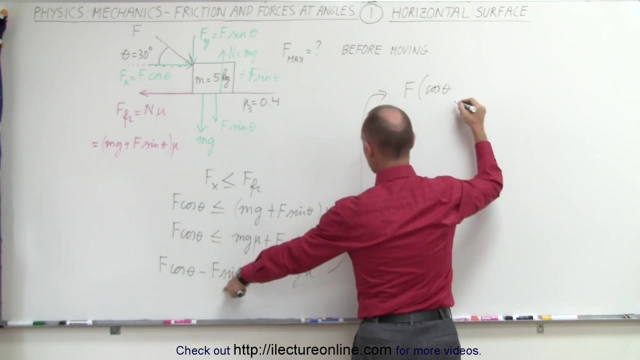 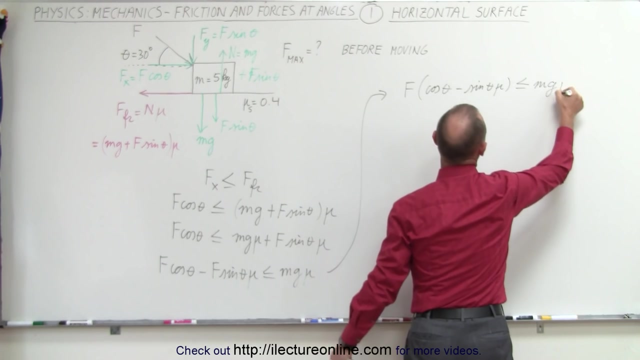 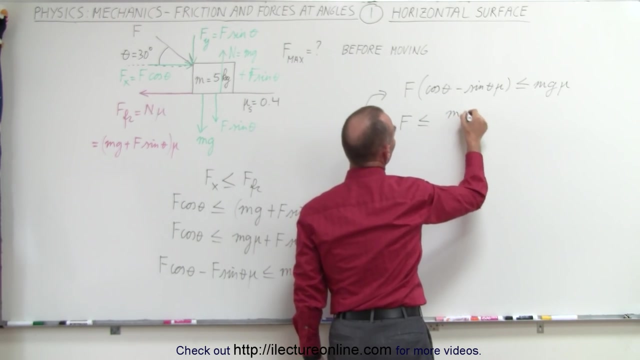 And then if we factor out an f- and let me move over here- we can then say that f times the cosine of theta minus the sine of theta times mu must be less than or equal to mg mu and then divide both sides by what's in the parentheses. that means f must be less than or equal to mg mu divided by the. 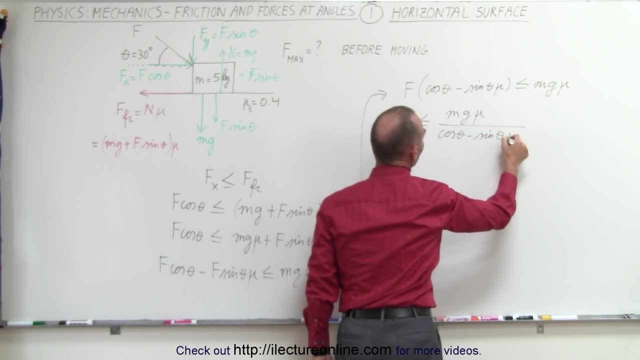 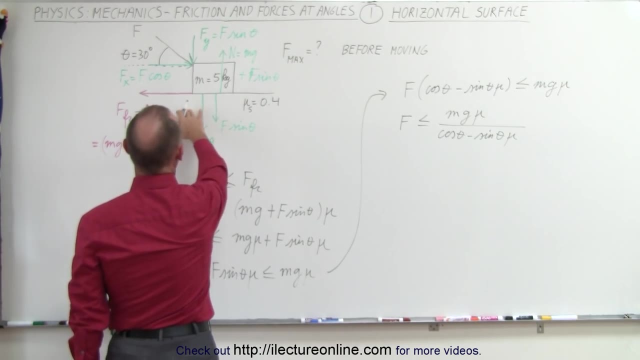 cosine of theta minus the sine of theta. Now we have to just plug in some numbers. and do we have numbers? Well, I have the mass, I have the coefficient of friction and I, oh well, f is what we're looking for. so I think we're good, so that. 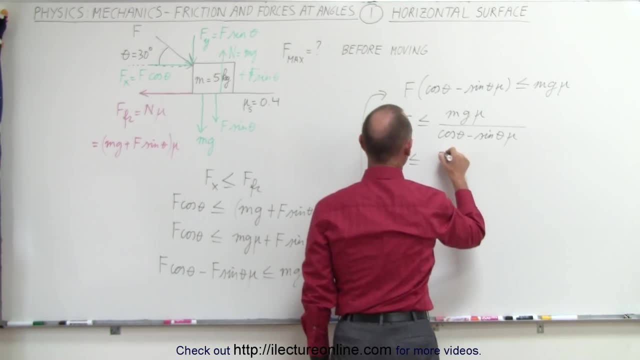 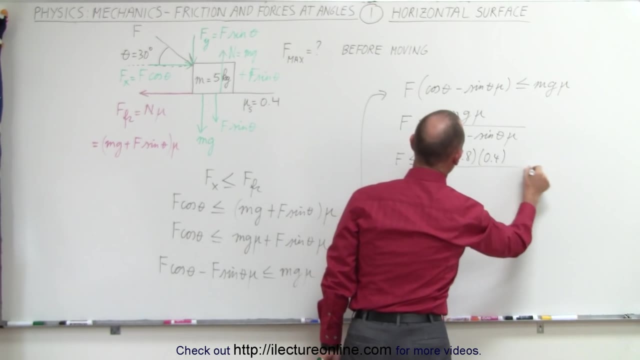 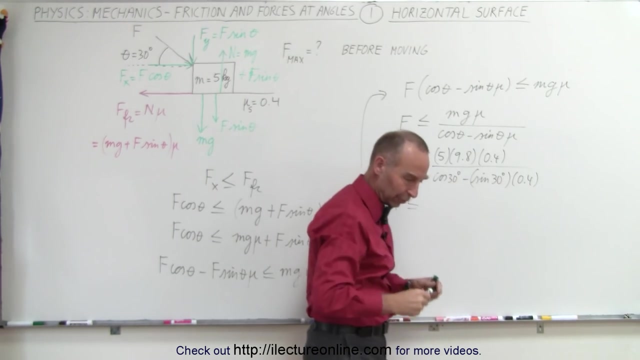 should be f less than or equal to 5 times 9.8 times that would be 0.4 divided by the cosine of 30 degrees minus the sine of 30 degrees multiplied times 0.4.. Alright, now we get a calculator and let's see what that force is equal to. so